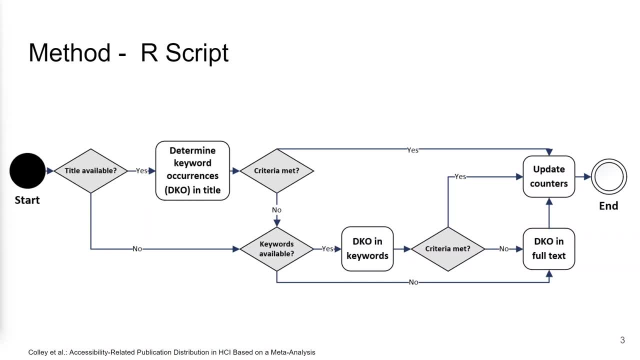 Our script then searched the keywords, first in the title, if the title was available via a field, then in the keywords, if available, and otherwise in the full text. We checked our approach with the data of assets. the ACM, SICK Access Conference on Computers and Accessibility from 2009 until 2019.. 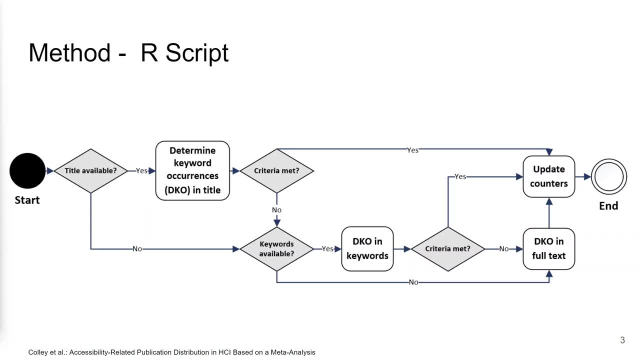 Which we categorized manually as well, After iteratively improving the process in the keywords. we then used this approach for 3617 field papers spanning assets: W4A, taxes, CHI, Auto-UI, MUM and WIST For the conferences other than assets. 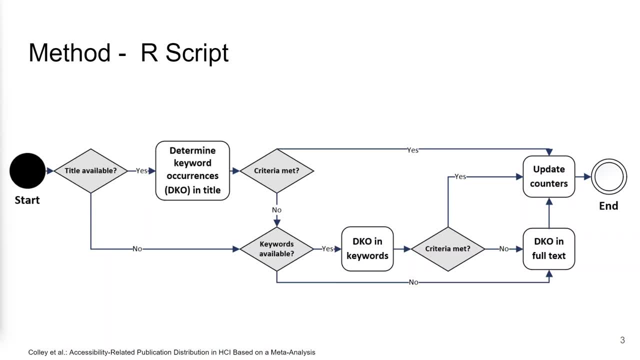 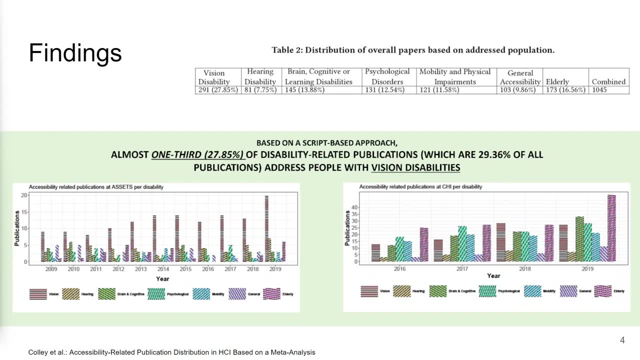 the time frame was 2016 until 2019.. The main finding is that 29.36% of all papers addressed the visual disabilities. Of these, 27.85% addressed visual disabilities. The focus on disabilities varied strongly between conferences. For example, at CHI, 20.49% of the papers addressed the. 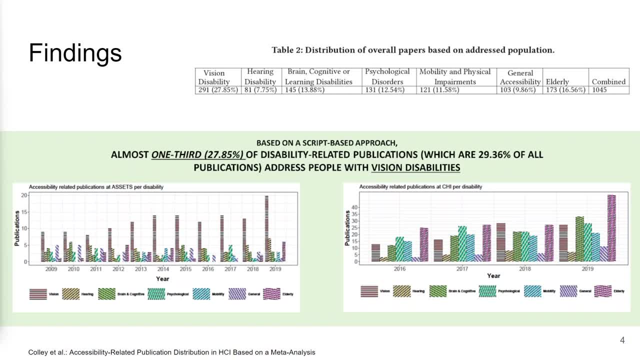 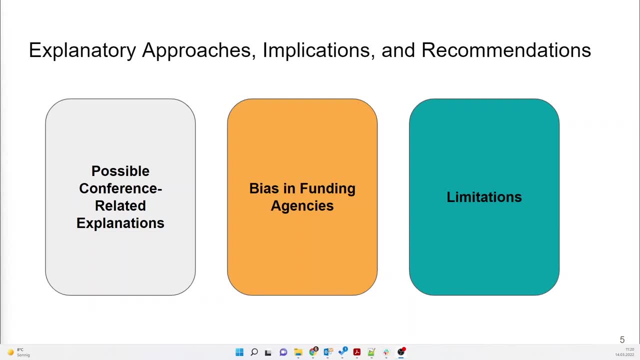 disabilities, while for Auto-UI this was only 2.2%. We tried to find explanatory approaches to the predominant focus on visual disabilities. We hypothesized that visual disabilities could be more tangible for researchers without disabilities, which we also discussed in our previous video. 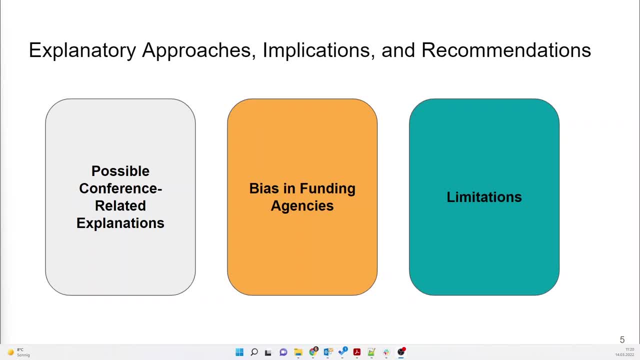 due to the prevalence of visual stimuli. However, work at CHI focused mostly on older adults and cognitive and psychological disabilities. Therefore, more research is necessary to unveil these trends. Regarding a bias in funding agencies, we found no data to support any bias. 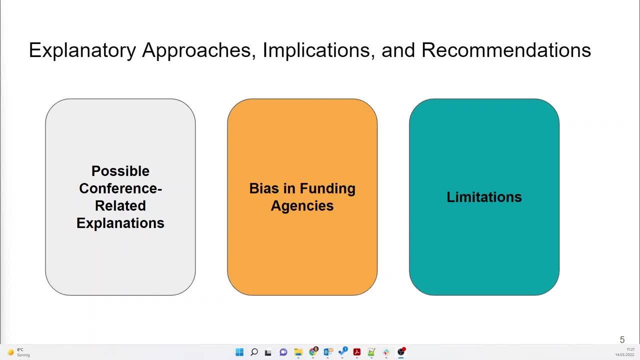 by analyzing 25 EU-funded research projects, 20 Canadian projects or Microsoft's AI for Accessibility program. Categorization is shaped by culture and worldview and itself shapes these. Thereby the employed script-based approach relied on terminology grounded in certain worldviews. 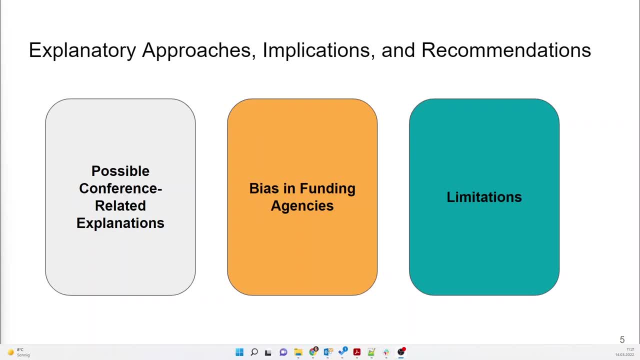 Additionally, such an approach is not perfect, as certain keywords could be missing or there could be potential conceptual overlap. Nonetheless, we believe that such an approach can help distinguish underlying patterns in HCI research. Thank you for your attention. Please subscribe to our channel. Feel free to contact me in case there are any questions.